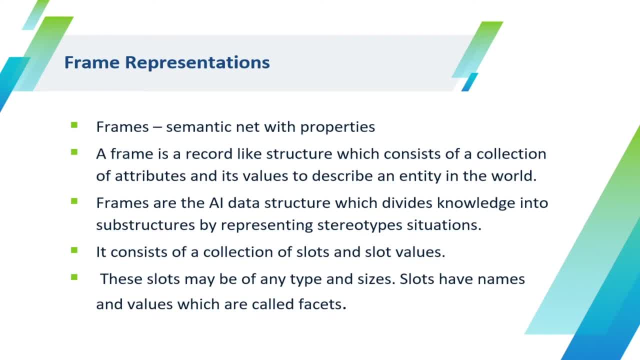 on I button, you will get the video link. Okay, So frame is semantic network with properties. A frame is a record, like structure, which consists of a collection of attributes and its value to describe the entity of the word In semantic network or partition semantic. 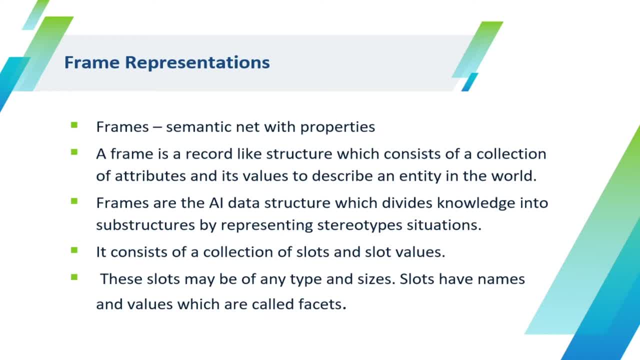 network or structural knowledge representations. we mostly concentrated on objects, different types of object and the relationship between the different different objects and entity. Okay, But in structural knowledge representations we are going to represent the object, but we are not going to represent the descriptions and we are not going to represent the different. 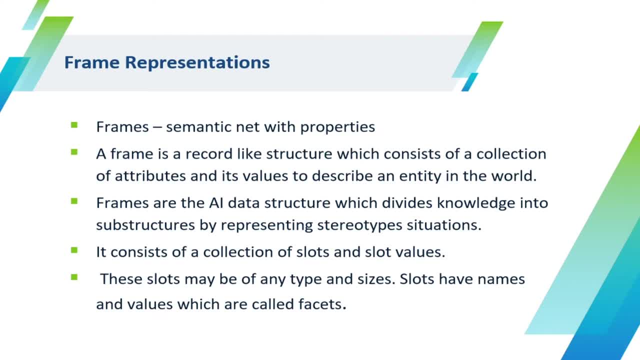 properties of that particular object. So we required a new representation technique. So that is the frame representation technique. I mean the semantic network we had and the partition semantic network we had. we could represent the object and its relationship, the relationship between different objects. 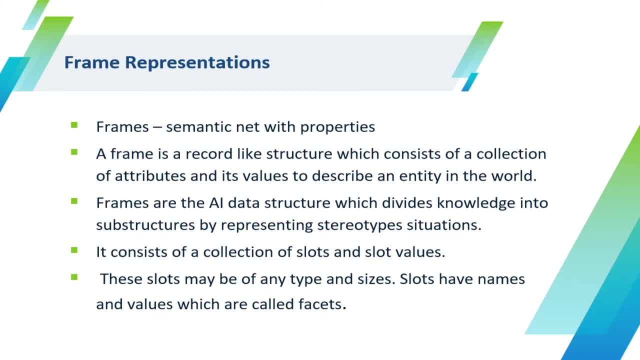 Right, So we have some new representation technique, And that is, we need some new representation technique. So this is how we will handle properties and descriptions of objects. You will need a frame representation technique which will handle properties and descriptions of objects. For example, if we want to remember the 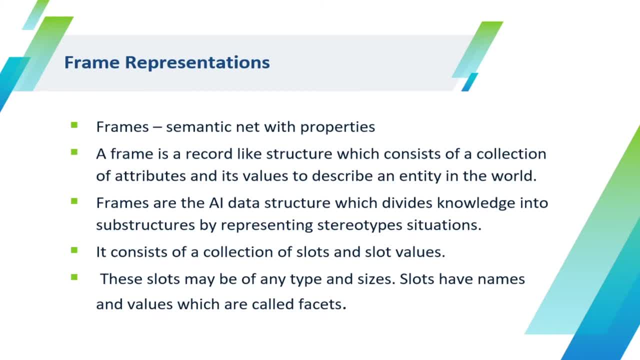 structure. it will handle the structure and the partition. So I will show you that will do the same. If you will understand this, you will know that the structure will handle properties and descriptions of objects also. All right record, like structure, which consists of collection of attributes and its value. 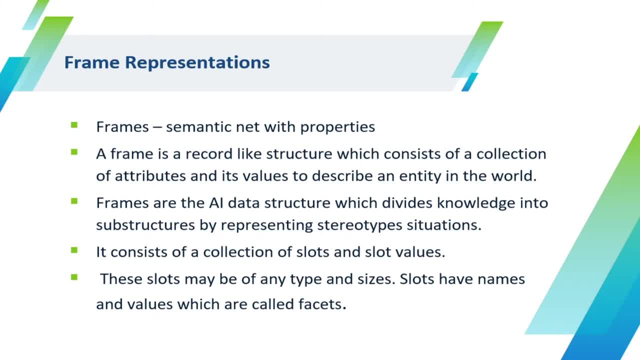 to the describe an entity in the world, but the frame make a hotel frame. it's a record, like structure. you have a up DCB object, DCB object and then musky properties can hook you or us kikun kusi values. okay, sorry, I've described the. 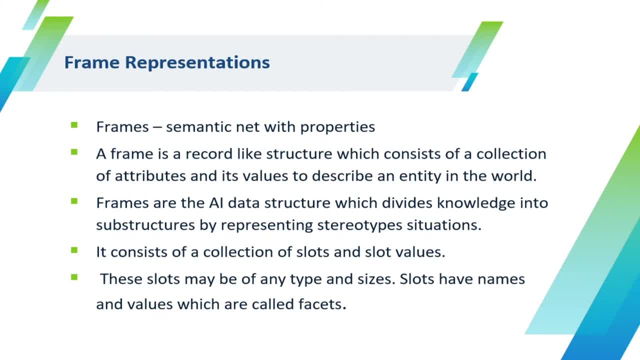 sector. frames are the AI data structure which divides the knowledge into the substructure by representing the stereotype situations. but the frame can determine how much data sector have. frame can determine how much objects kujo be data have a properly represent kuseki properties could represent kuseki events are generate. okay, was sorry, I'm represent kuseki Oscar data. or 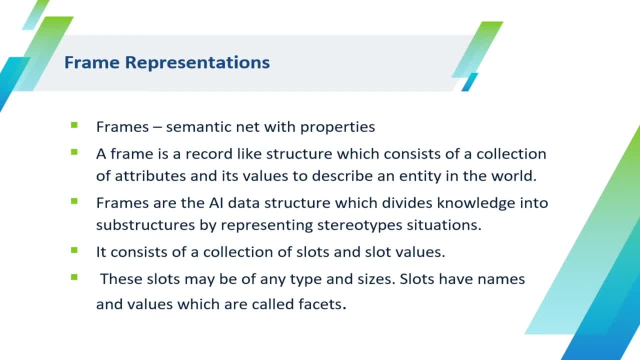 us k events. kya hoge was sorry. I'm represent kuseki. a hum example met some change. it consists of collection of slots and slot values. slot is nothing about the property and slot values is nothing, nothing about the values. I'm the object oriented, where paradigms can then make the cow ahead, classes and 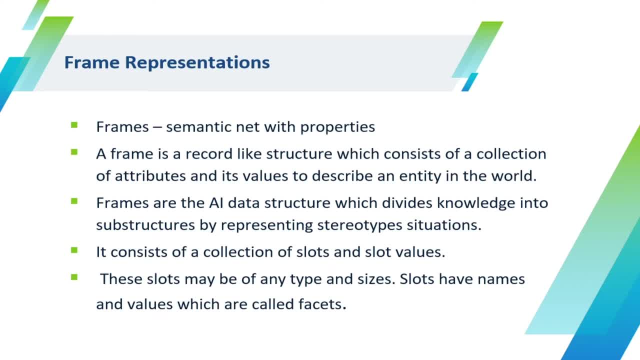 collection of data in the frame. we can represent the data in the frame and class diagrams. class diagram can determine a sautee individual classes. of the individual classes. may I'm kiss the sapsic uski properties could describe, describe, cut it where I'm. are out there uski properties or uski values? 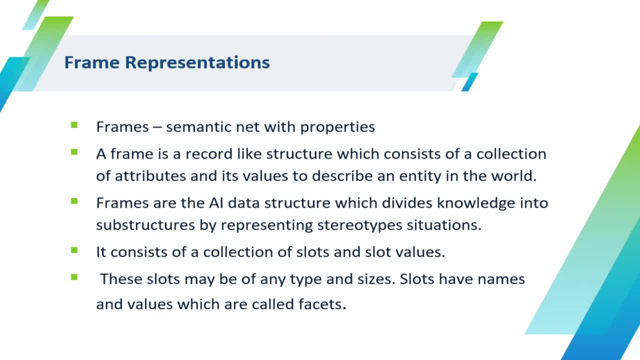 similarly. hum, yeah, I'm a knowledge. represent carnavala head job be object huga was maybe hum uski to properties who give us k according hum muski values stored parker pangae. these slots may be any type and any size. slot, seven names and values which will call as facets but love. 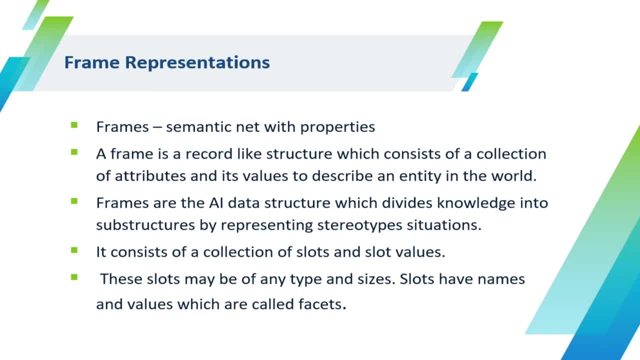 kill me a frame. soul kill frames came under my job. you are values, oh, good job. you soge Jaubi feelers okay was kicked, which not okay, or skin under my kuch. one values only valley here chicken yes, aumple mapo sandwich about the slot ke. 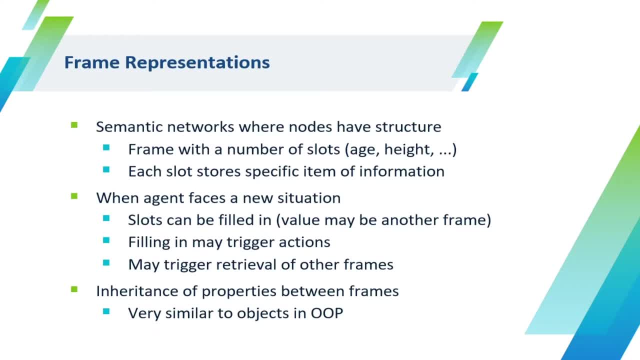 all that filler keota. okay, so semantic network where node have a structure, hum, the semantic network made it kaki, wahaipan, northo today. or different, different nodes ke vich my relationships OTA. but frame alguna vala, frame with a number of slots, frame can better me. for example, could object head what I'm going to do to change the frame, number of slots or object or object like this is a good idea. 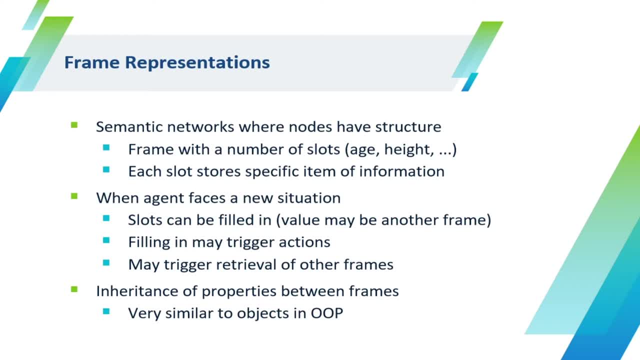 There will be different properties in the object. for example, man can have a property of age, height, weight. We can define its properties in this way, So human being can have an age, height and property. So there will be a particular value of age and a particular value of height. 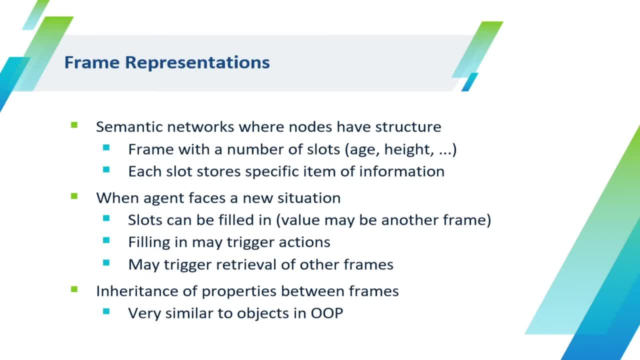 So age is a property and the value will be called as filler and property is called as slots. These slots store a specific item of information. When agent faces a new situation, slots can be filled in. a value may be from another frame Means if we have a class and there is a new situation, then it can take reference of another frame. 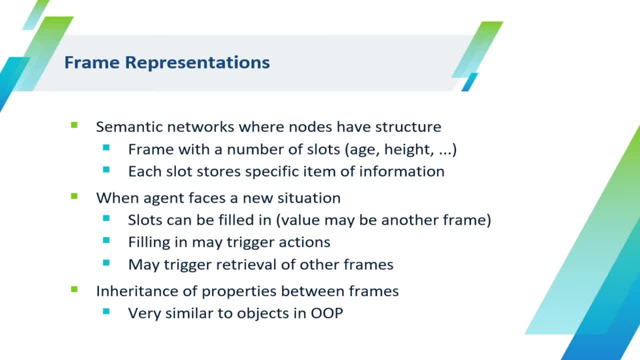 Filling in. made trigger are actions. Made trigger are retrieval of other frames. We will see this example. In this example we will understand how another frame will be referenced. Inheritance of properties between the frames is very similar to the object in object-oriented paradigms. 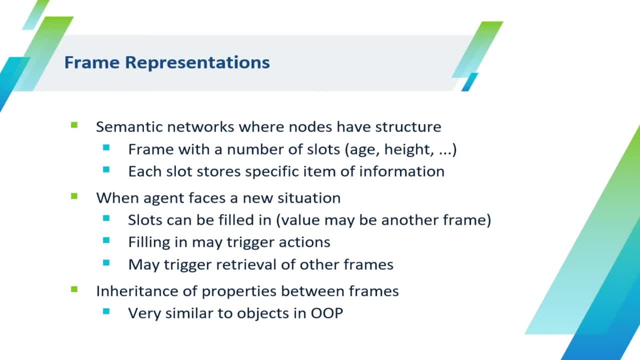 So the way we have studied class diagrams in object-oriented paradigms, Similarly these are frame representations. The way we use classes in class diagram, we will use frames there. What will happen in frames? There will be slots and fillers in frames. It is very simple. 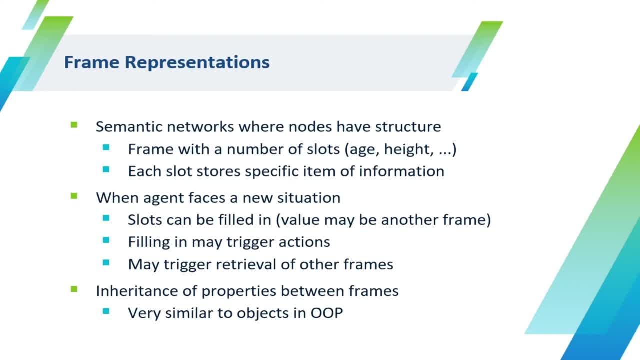 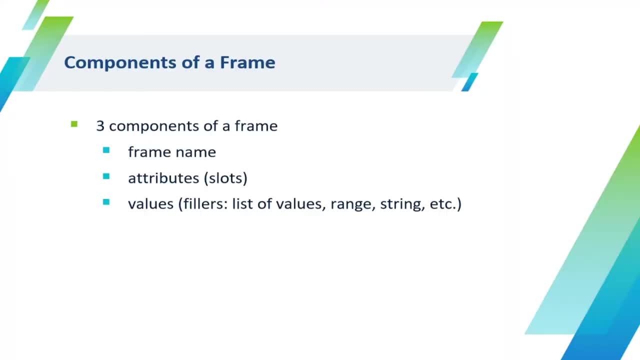 We are going to represent the class with frames, The same thing that we call frame representations. You will understand in the example. So basically frame has three components: Frame name attribute- that is also called slots- And values- it is called as fillers, The list of values, range, string, etc. 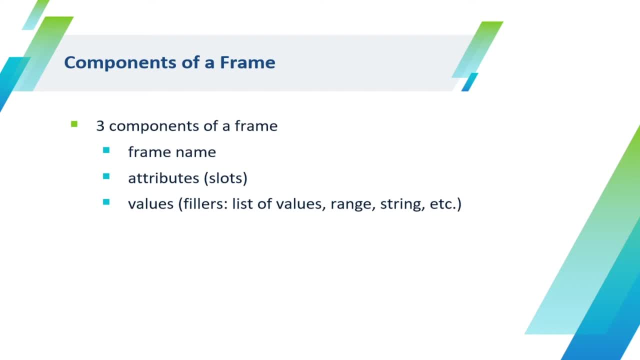 As we have seen in class, class has a name. The properties or attributes in class are the attributes and values of that attribute. So the attribute is called slots And the values are called fillers. So we will see the examples, How a frame is made. 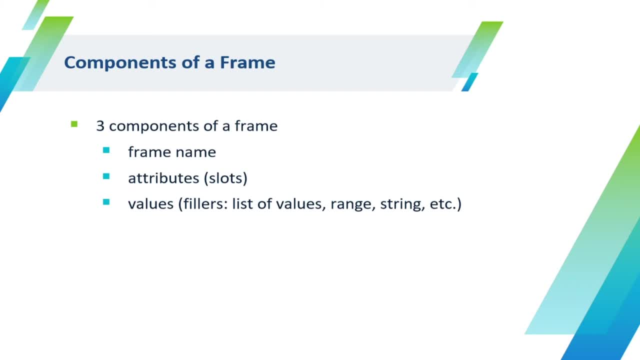 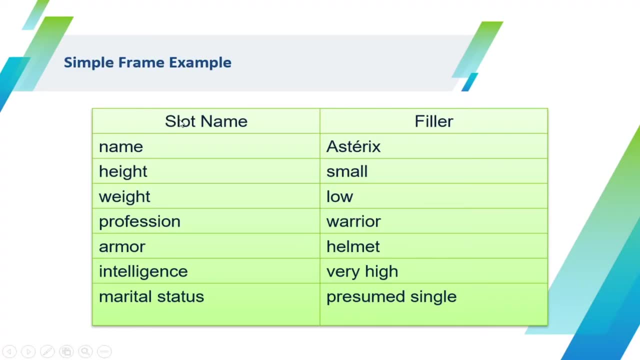 For example, in our class diagram we used class. Similarly, we will make the frame So simple. example of frame. So that is a slot name, filler name, For example. we have a property named name, So name can be anything, So its values will be according to the name. 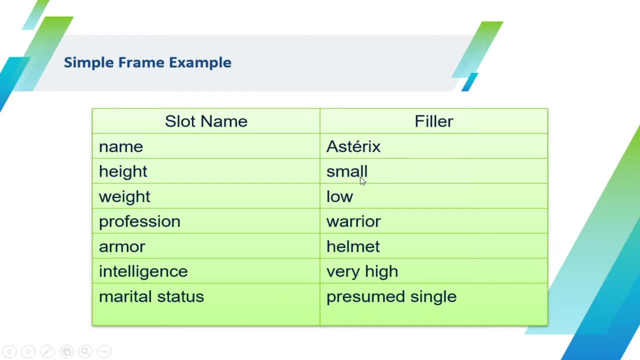 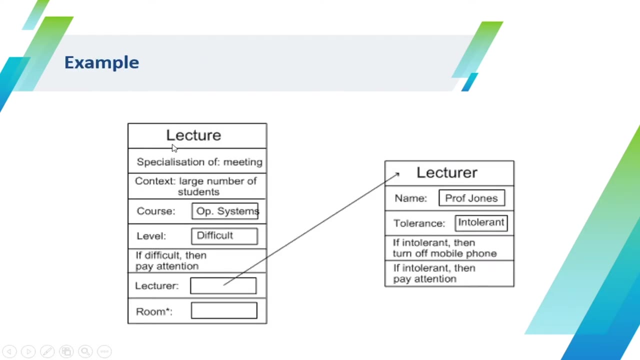 Height: small, Medium Height. Weight: low, Mid-range, Heavy Professional warrior. So this is nothing about the properties And this is nothing about your values. So we will see an example of lecture. So what will happen in the lecture? What is the lecture about? 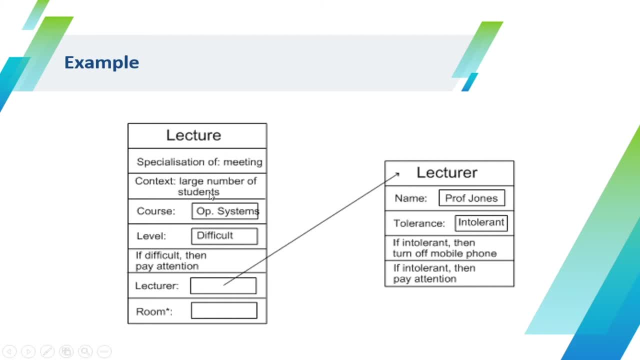 The lecture is about meeting. What is the context? Large number of students. We are taking lecture for all number of students. What is the lecture for Course? its operating system? What is the level? Difficult, If difficult, then pay attentions. So this is nothing about the descriptions of lecture. 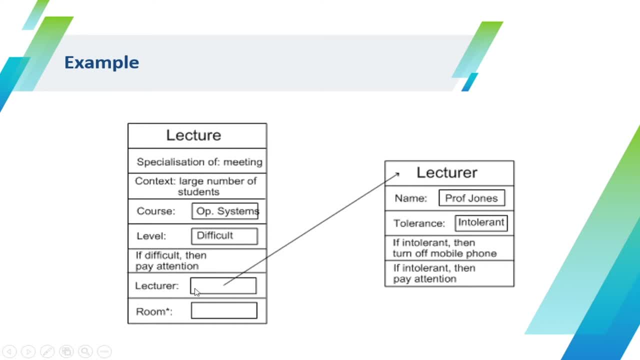 Now, who is taking the lecture? If someone is taking the lecture, then it should be the name of the faculty. So what does the lecture do? It represents another frame, As you can see. lecturer, Lecturer name: Professor Johns. Tolerance intolerant. 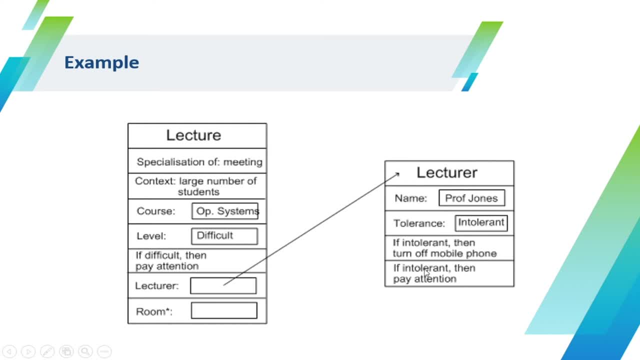 If intolerant, then turn off the mobile phone. If intolerant, then pay attentions. So this is how we defined lecturer. So this is a simple frame. If you know the class diagram, In the class diagram we used to make classes in the same way. 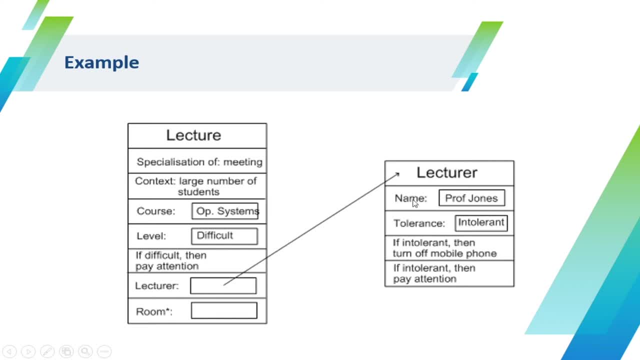 For example, we used to give the name of the class at the top And here we used to represent its different properties and different values. In the same way, in the frames, Here the name of the frame will be the name of the frame. Here slots will be there and its fillers will be the values. 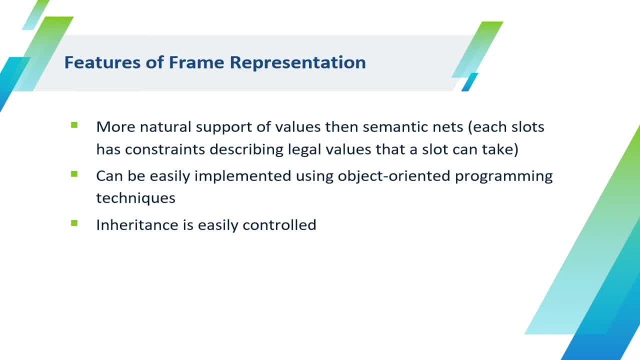 So this is a simple example of lecturer. So what is the feature of frame? This is the feature of frame representations. Features of a frame representation: More natural support of the values than the semantic net. Each slot has a constraint describing the legal values that slot can take. 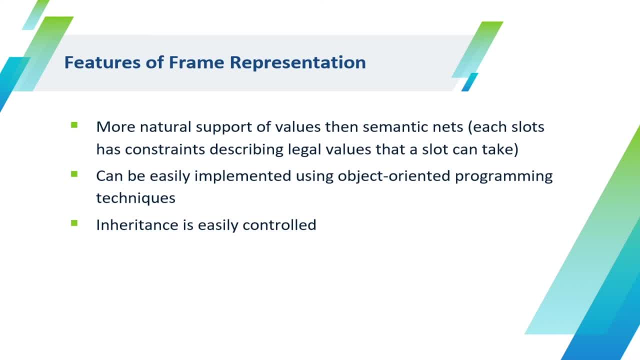 Means whatever properties are there in the frame. There will be some values of those properties And you can set it according to the conditions. For example, there will be a range, a legal range. You can set that value. For example, height, Height- never be in negative. 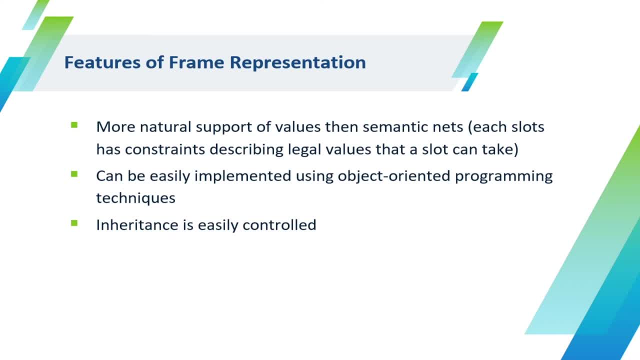 Age never be in negative, So you can set the conditions in this way- Can be easily implemented using object oriented programming technique. The way we studied the class diagram. Our class diagram is also a frame representation technique. Inheritance is easily controlled Using frame representations. we can control the inheritance properly. 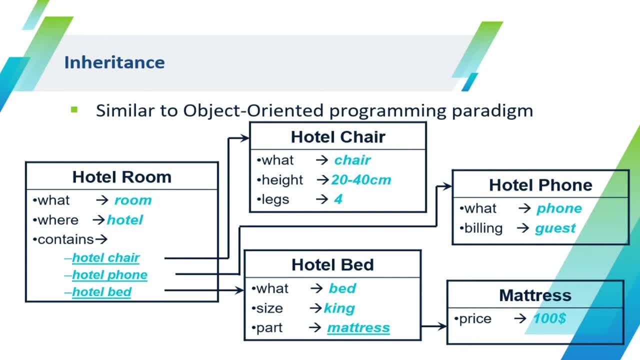 So these are the features. Let's see one more example Similar to object oriented programming. For example, there is a one frame hotel room, What It's a room Where Room in hotel. What Hotel room contains what? Hotel chair, Hotel phone And hotel bed. 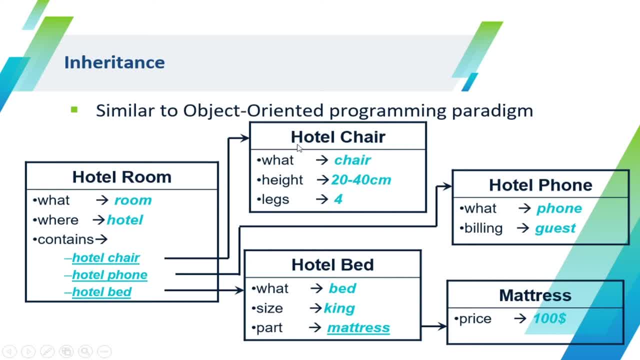 Now, what is hotel chair? Hotel chair references to another frame that is hotel chair. What It's? a chair Height is 20 to 40 cm. It has four legs. Hotel chair has four legs. Okay, Now hotel room contains hotel phone also, So it describes hotel phone. 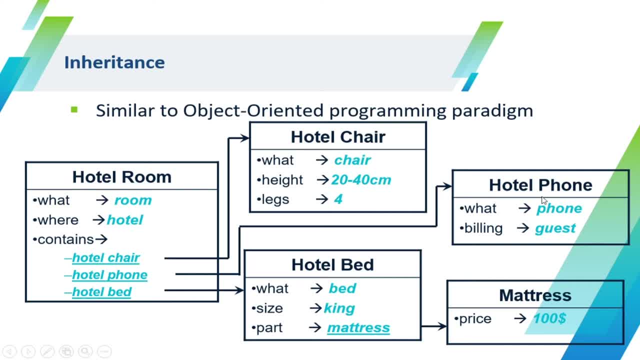 What It's a phone Billing. While we use a phone, We have to pay. This is billed by the guest. Okay, Hotel bed. It's a hotel bed. What It's a bed Size is king size. Hotel bed has a part that is mattress. Now, what is mattress? 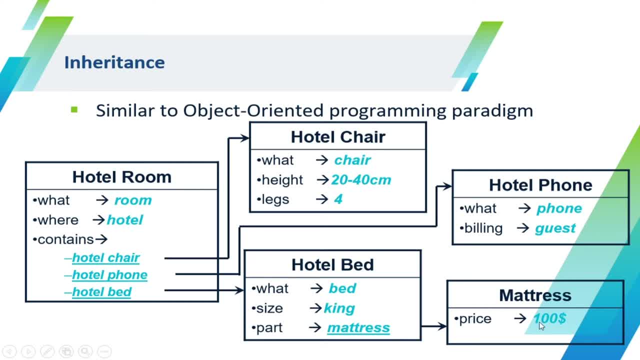 Mattress is having a price, Let's say $100. So this is nothing about your different frames, Which is reference to another frame And which will trigger another frame And which will describe another frame, Another property And other descriptions. Okay, So similar to object oriented Like a class diagram. 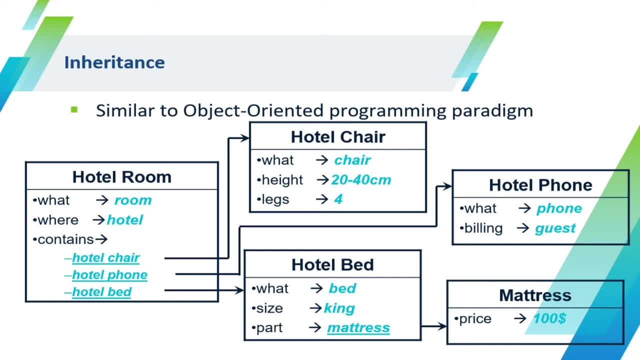 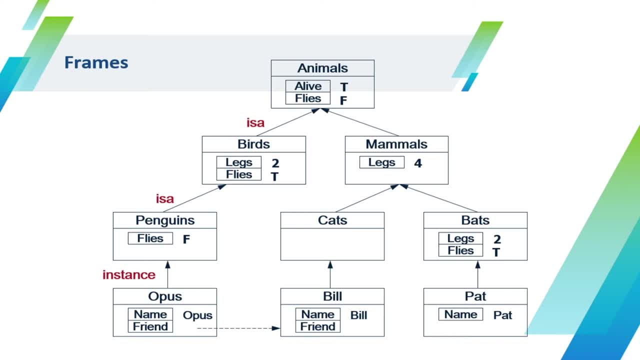 We are going to represent our knowledge Using frame representation technique. Okay, So we also have another example. This example represent the inheritance. Okay, So we have a top most frame here: Animal Alive. It's true, Animal can fly, buffer. So this is the basic frame, This is the parent frame. Okay, a bird is an animal. bird is an animal. 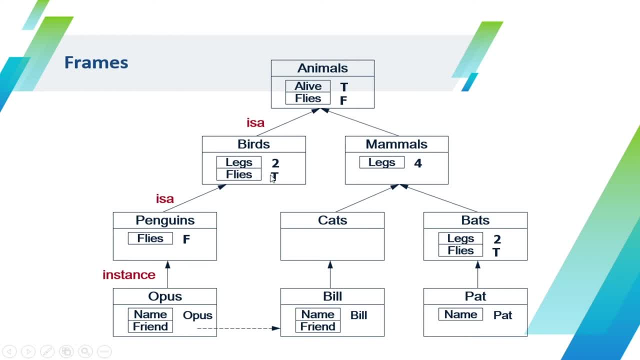 Leg, it's a two Flies. Yes, it's true. So what is an animal who can fly mammals? It has a four leg. It has a two leg also. Okay, so legs, So legs is a property and for it's a value. 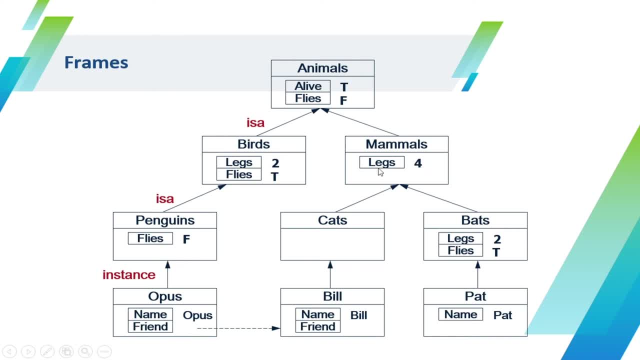 Okay, it is called as filler. legs can in in the term of frame. We can say that legs is a slot and the bar its value, for it's called as fillers. Okay, so pigments. Pigments can fly. It's a false instance of opus opus. It's object of pigments. 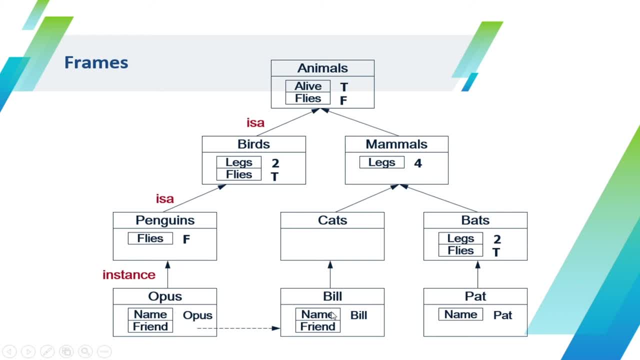 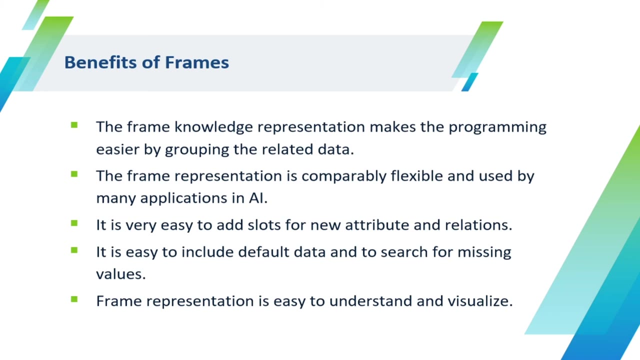 Okay, so the name is opus, Fred is bill, and now who is bill? bill is a cat, So similarly, we can represent the inheritance properly using the frame representations. Now the what is the benefits of frames? the frame, now the frame. knowledge representations make the programming easier by 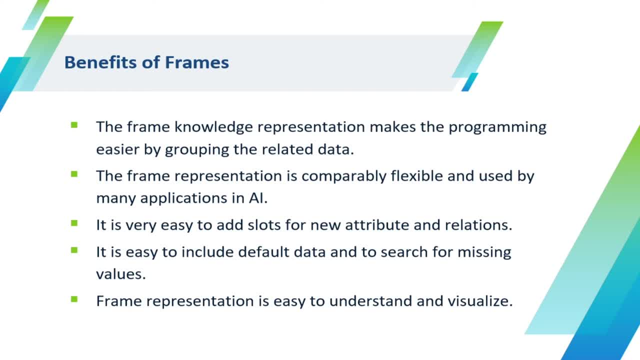 grouping. the related data Frame representation is comparably flexible and used by a many applications in artificial intelligence. Okay, so it is very easy to add slots for a new attribute under the relationship and a different relationships. It is easy to include Default data and to search for the missing values whenever we require some missing values.